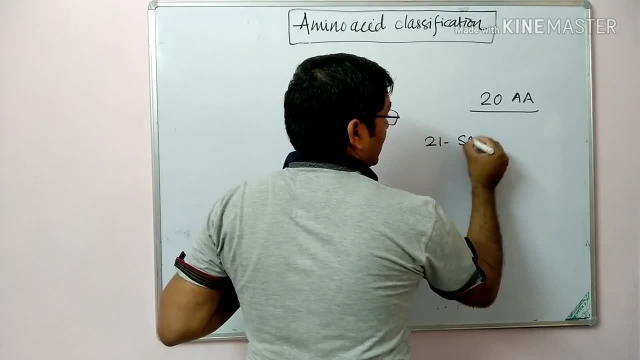 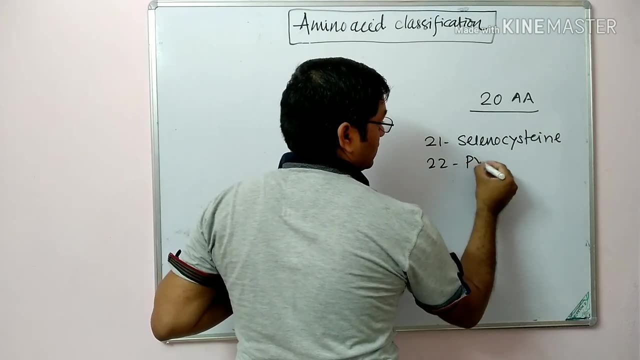 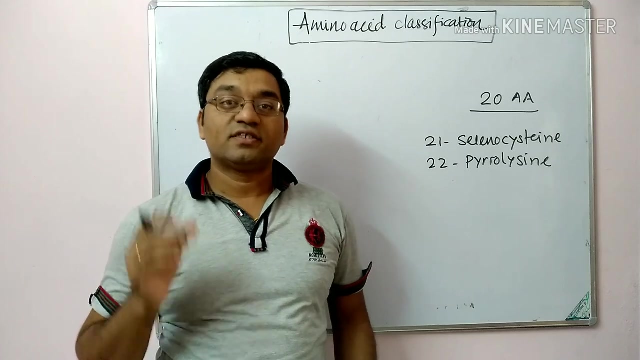 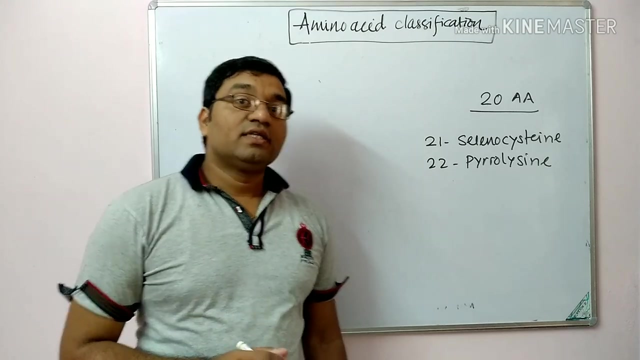 of 21st amino acid, that is selenoxysteine, and 22nd is also there, that is pyrolysin. So there are 22 amino acids which gets incorporated into the protein and helps in the protein synthesis. Now we will see the classification of amino acid. They are classified on the: 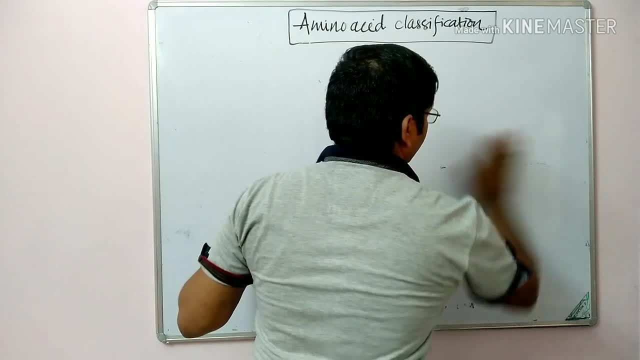 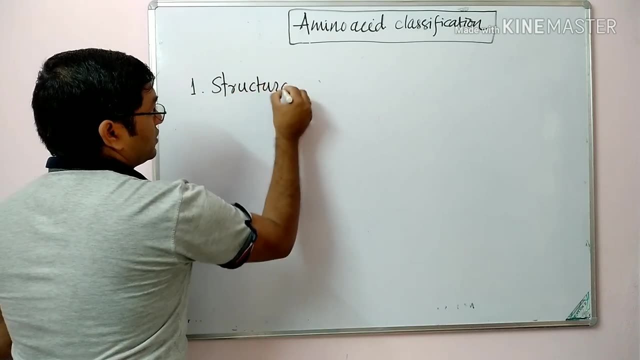 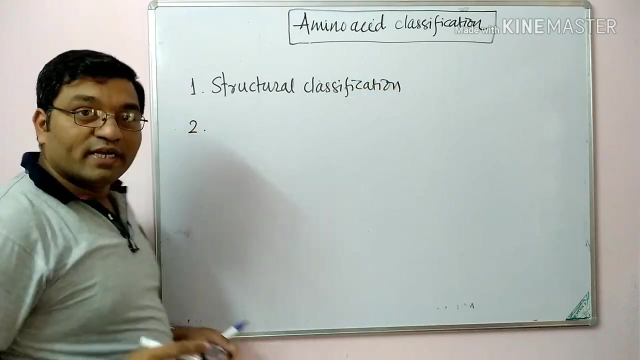 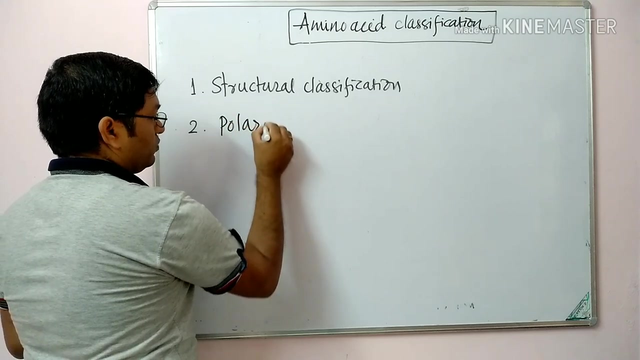 basis of 4 things, or on the basis of 4 ways they are classified. The first one is known as the structural classification. Second, it is based on the solubility, that is, polar and non-polar Means based on polarity Hydrophilic amino acids, they are known as. 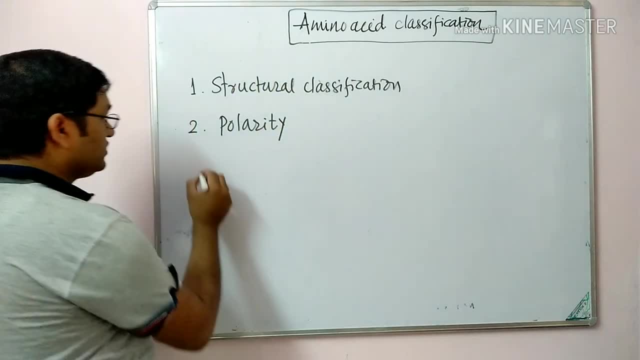 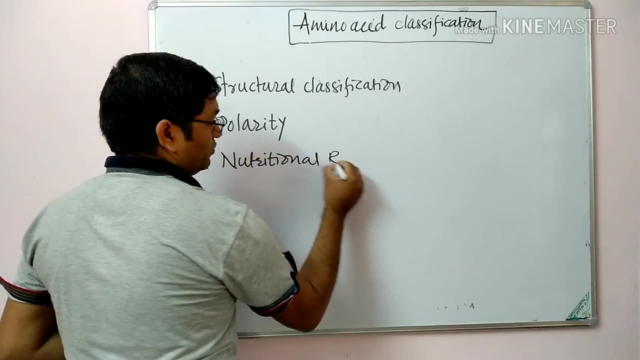 polar and hydrophobic amino acids. they are known as non-polar amino acids. Then, third one is the nutritional classification. So the first one is known as the structural classification, The second one is the nutritional requirement And fourth one is the metabolic fate Depending. 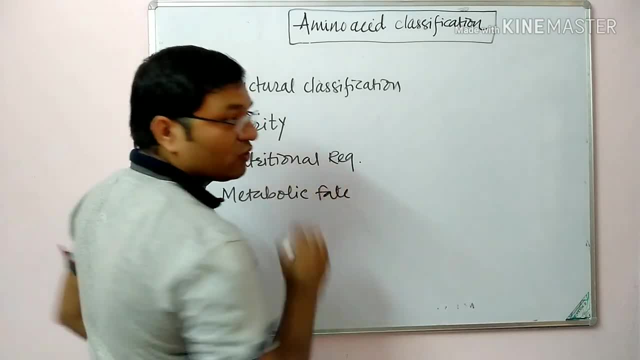 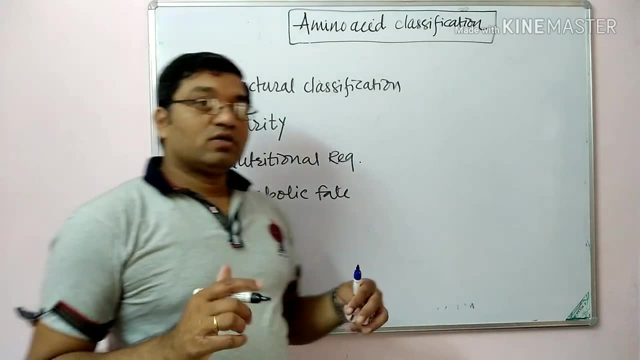 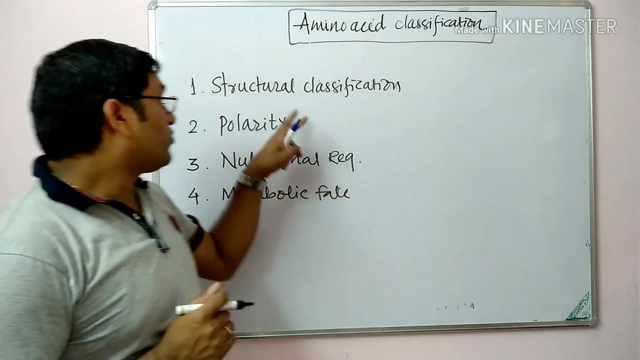 on their metabolic fate. they are known as glucogenic or ketogenic, or both glucogenic and ketogenic. So if you answer this question in the viva, if there is a question in the viva, classify the amino acid. So you should tell these 4 points They are classified on. 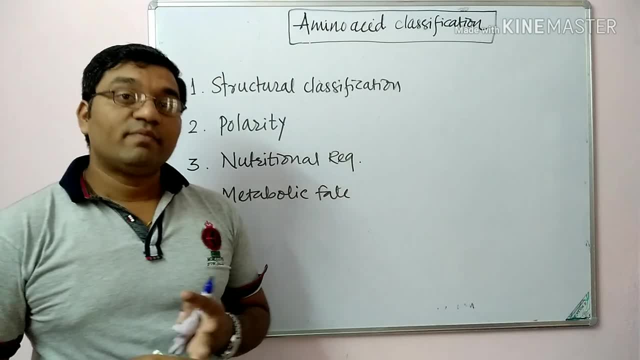 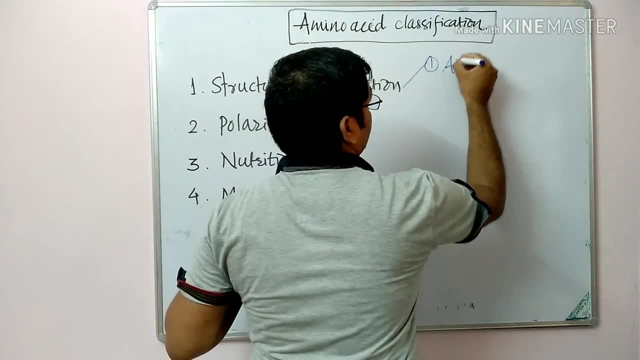 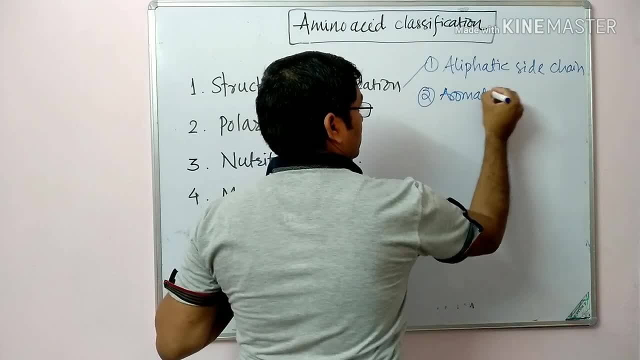 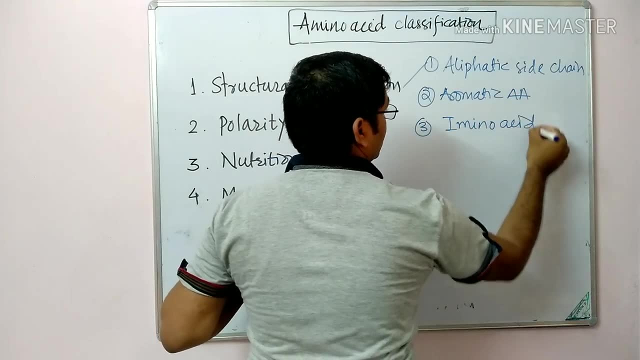 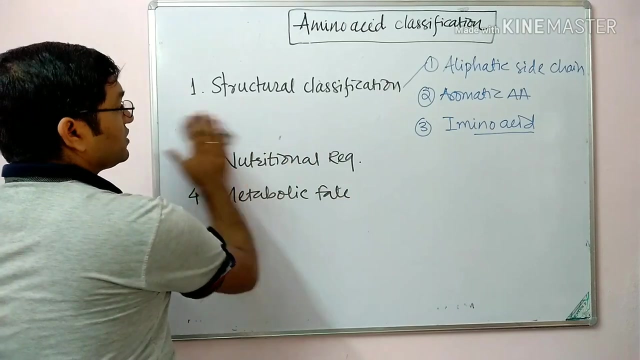 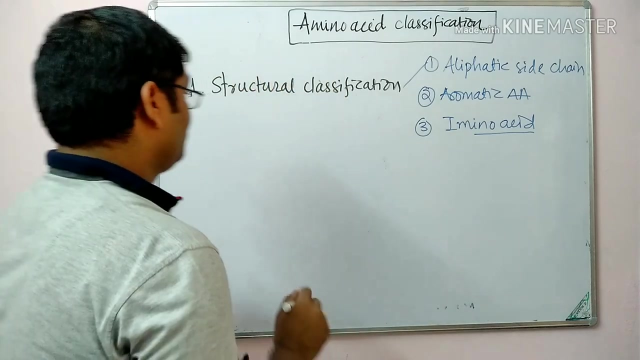 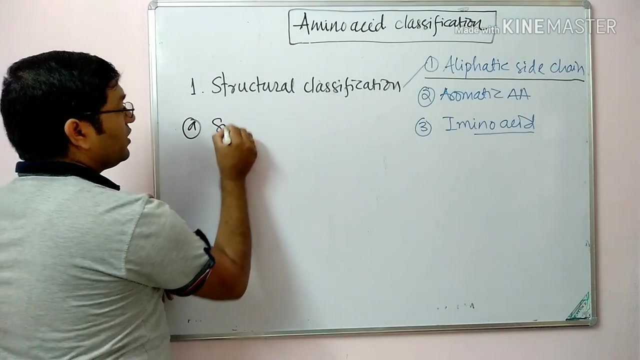 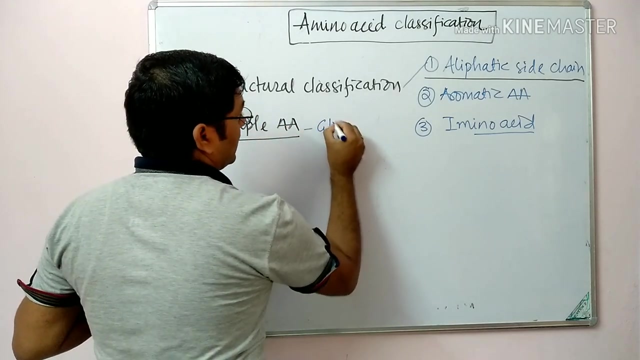 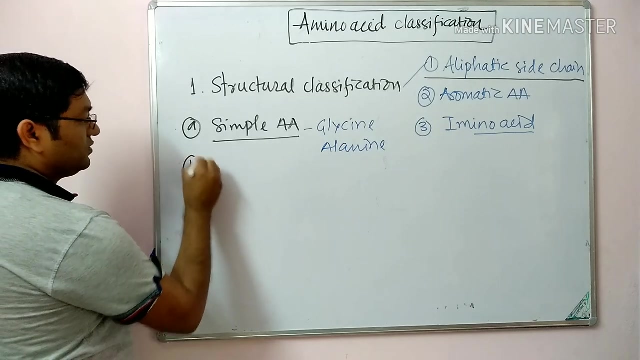 classified on the basis of their structural classification. So you should tell these 4 points. They are classified on the basis of their structural classification. This is section four. Each minor acid has its own stopping point: simple amino acids. This includes glycine and alanine. Second one is the branch chain. 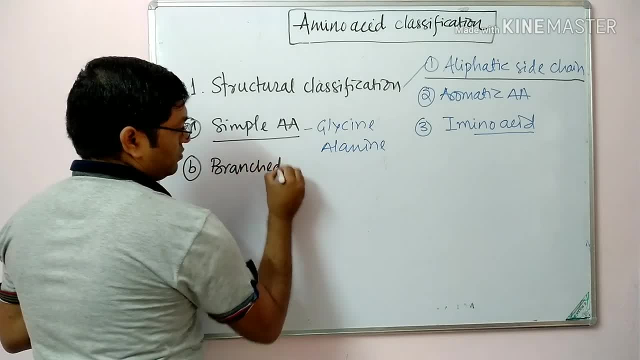 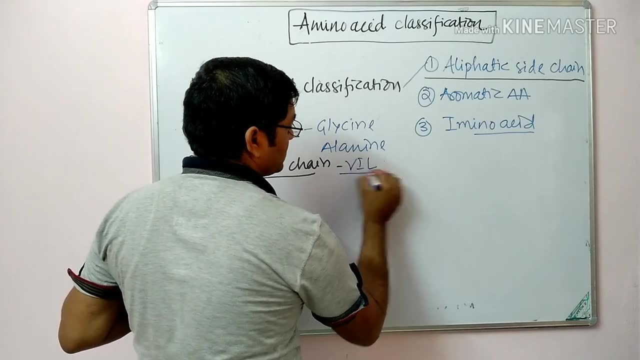 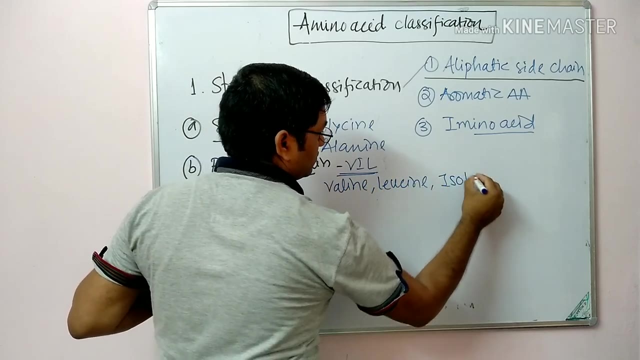 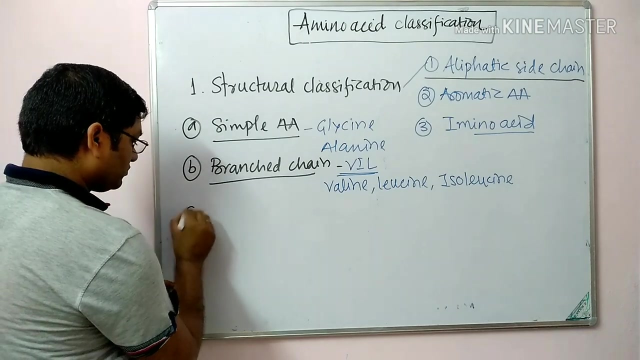 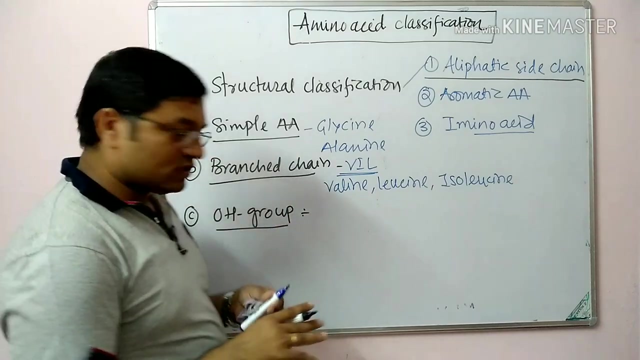 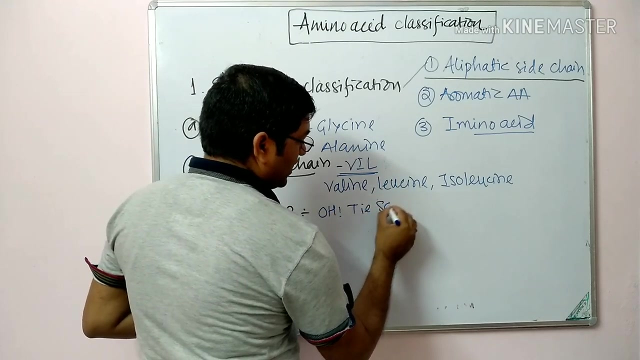 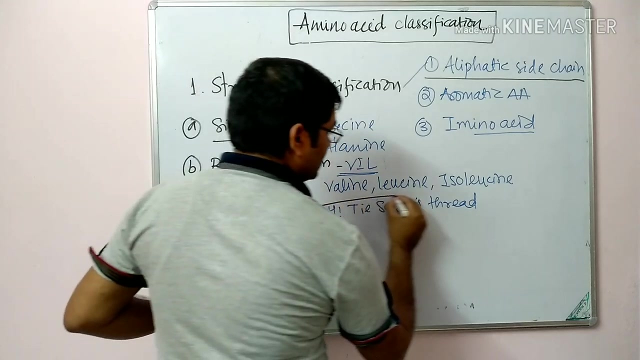 amino acid. This includes, that is, VIL, means valine leucine and isoleucine. These are branch chain amino acids. Then third one is the OEH group containing: There is mnemonic for this. The mnemonic is Systemic, naturally treated. 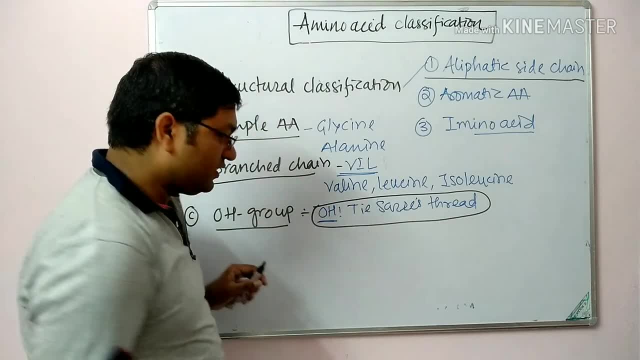 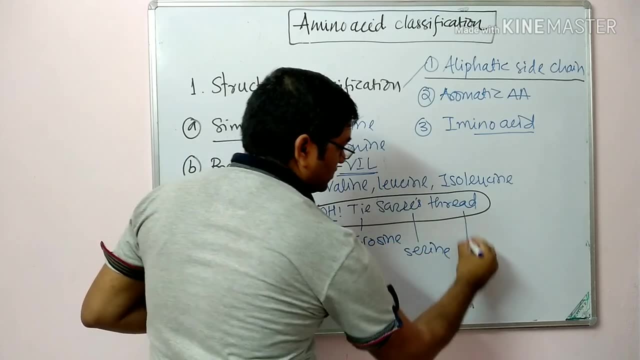 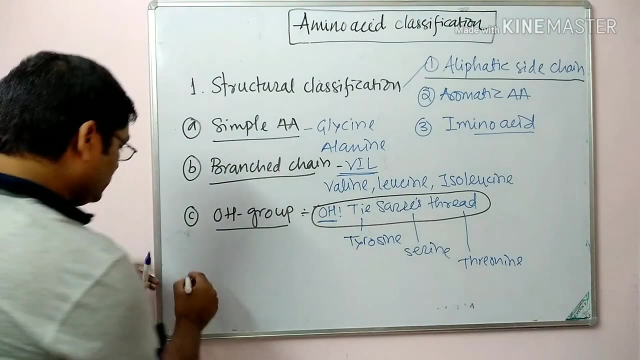 compound O. O means OEH group containing. This is from tyrosine, cryopropylene, Mass, Närieve, Haszo, ated. This one is for serine And this is threonine. So these are OH group containing amino acids. Then the simple ones, that is sulfur containing amino acid. These are methionine, cysteine and cysteine. Cysteine is formed by the two molecules of cysteine, So methionine and cysteine belongs to the sulfur containing amino acid. Then fifth, one, Simple one, that is, acidic amino acids. 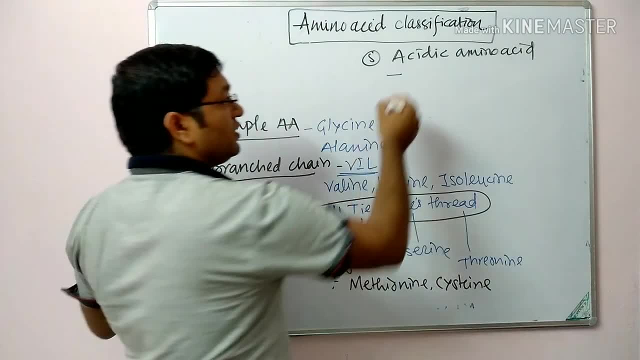 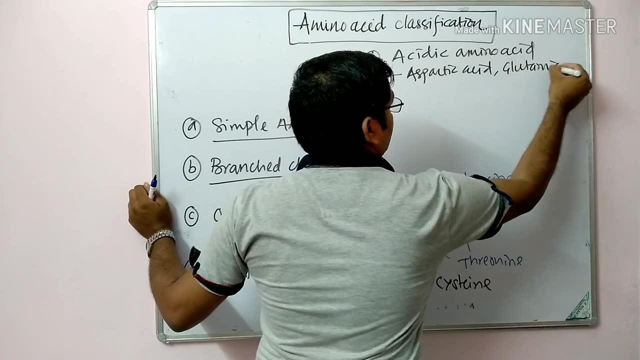 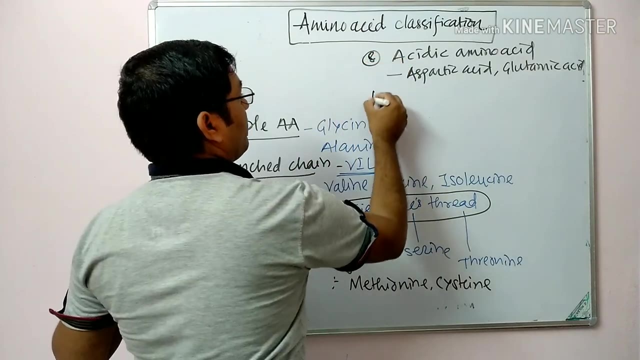 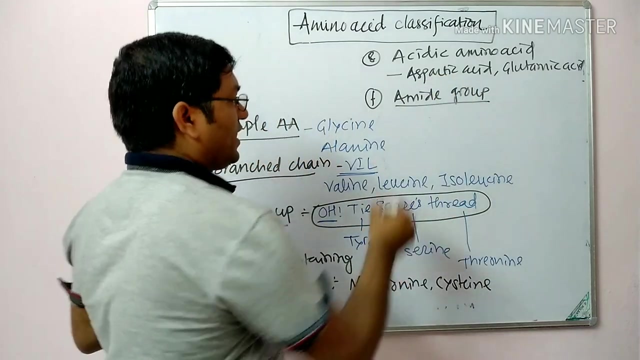 You know the name suggests the acidic amino acid, that is, aspartic acid and glutamic acid. Then first, second, third, fourth, that is E, F, That is amino acid with amide group, The amide group, that is asparagine and glutamine. 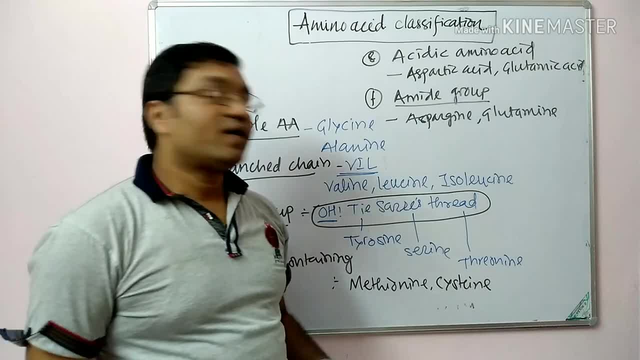 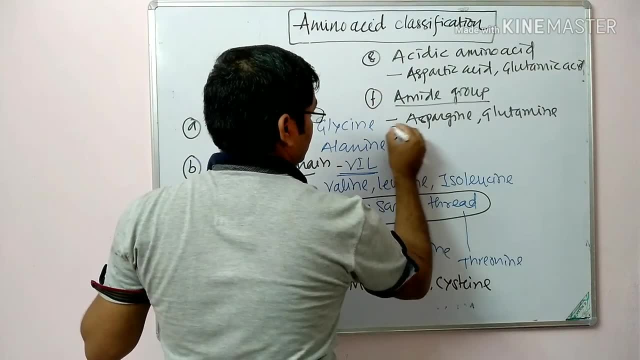 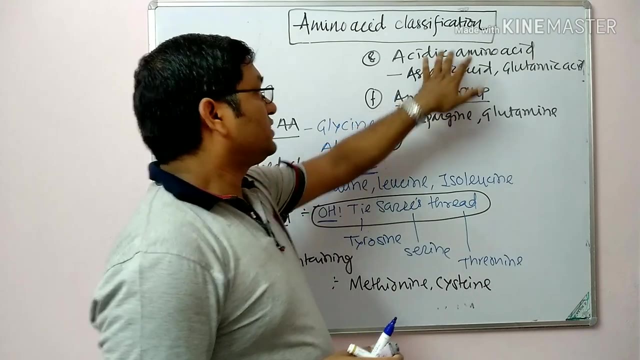 These are acetic amino acid, aspartic acid, glutamic acid, The amino acid with amide group. these are the asparagine and glutamine. The one is left, That is first. one is the simple, then branch chain, then OH group, containing then sulfur, containing then acetic amino acids, amide group containing amino acids and basic amino acids. 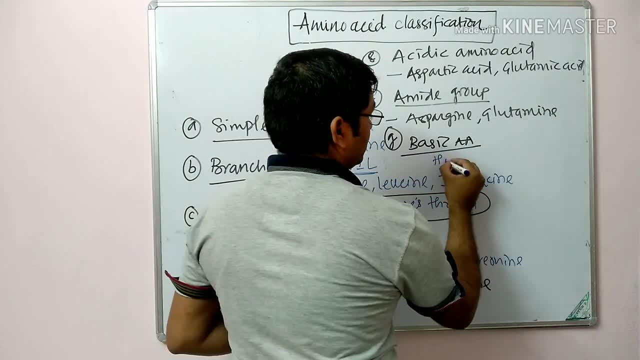 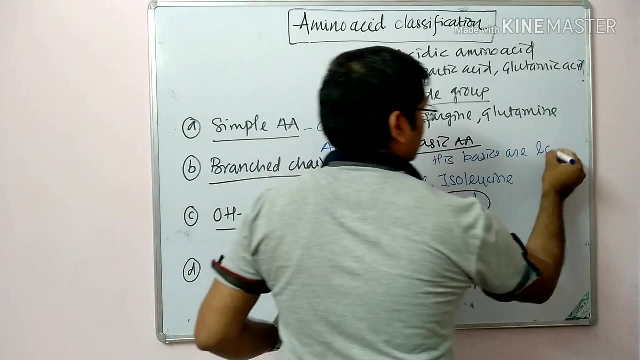 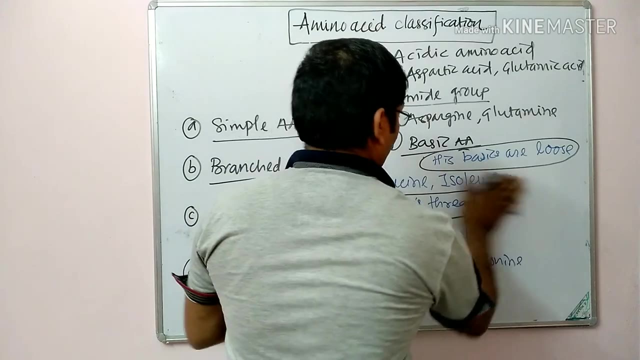 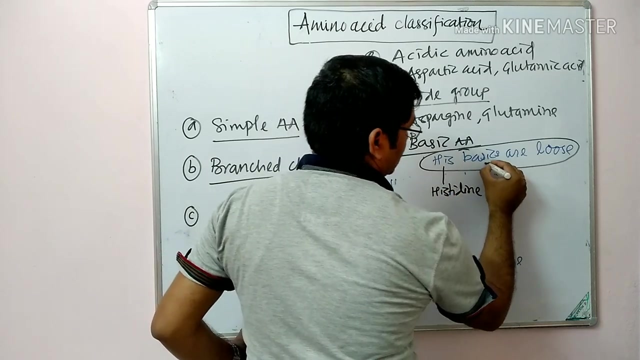 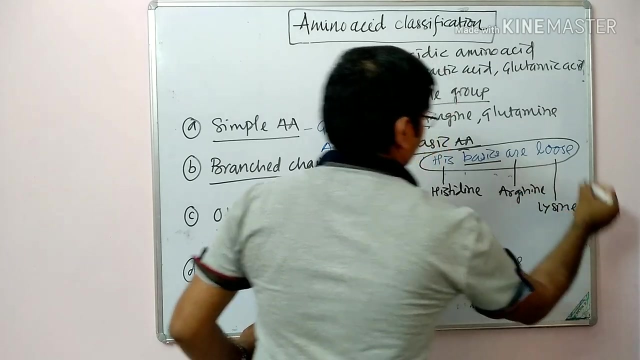 There is pneumonic for basic amino acid. that is, his basic are loose, His basics are loose. This HIS means histidine. these are the basic amino acids: arginine and lysine. So these are the basic amino acids. So these are the amino acids with aliphatic side chain. 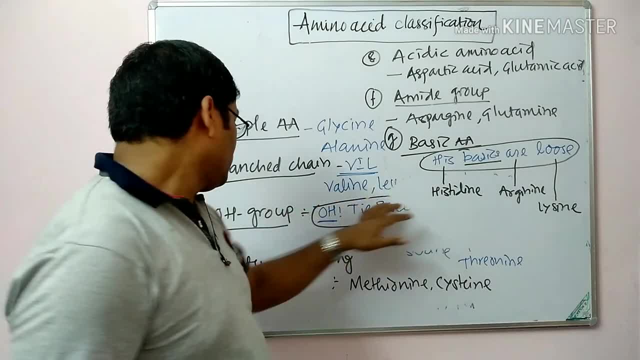 The first one is the simple glycine, alanine, then branch chain, valine, isoleucine, leucine, then OH group containing, that is, tyrosine, serine and threonine, then sulfur containing. Cysteine, cysteine, methionine, then acetic amino acid, aspartic acid, glutamic acid containing amide group, that is asparagine, glutamine, and basic amino acid, that is histidine, arginine and lysine. So these are the amino acids with aliphatic side chain, Coming to the second one, that is, aromatic amino acids In aromatic amino acids, The first one is the phenylalanine, second one is the tyrosine, then the aromatic amino acids with heterocyclic ring. 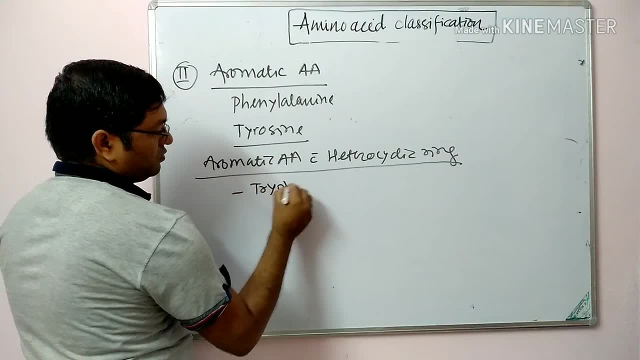 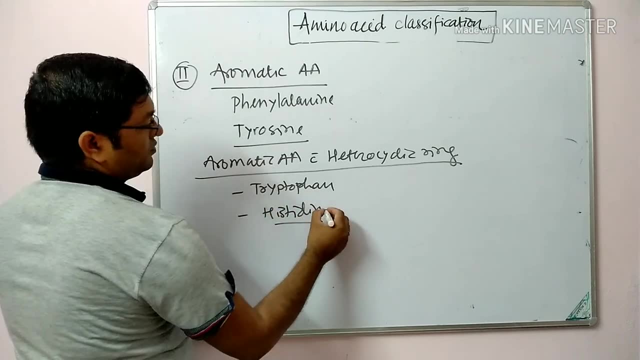 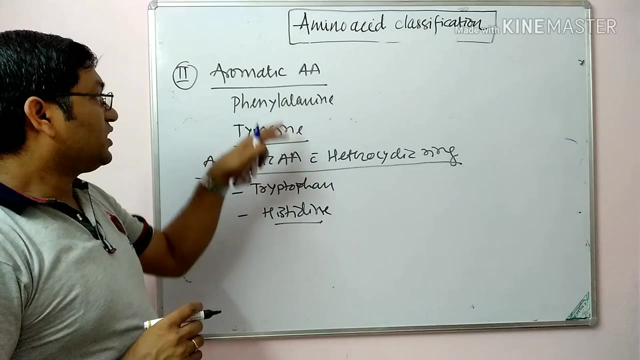 This includes tryptophan and histidine, So this one is the basic amino acid And also aromatic amino acid with heterocyclic ring. So these are the aromatic amino acids: phenylalanine, tyrosine, tryptophan and histidine. 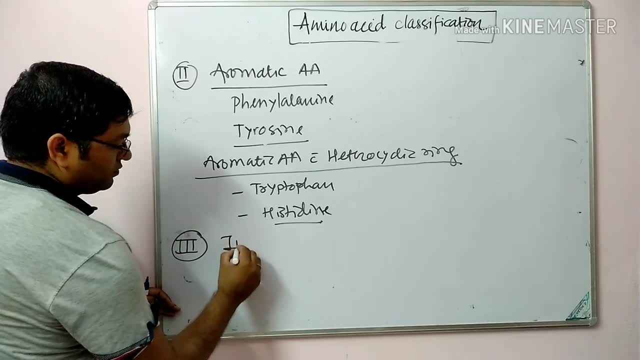 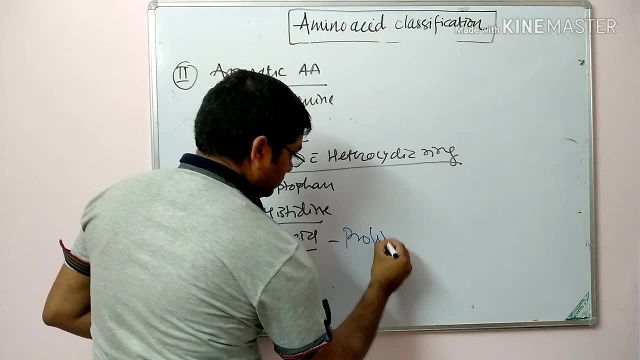 And the third one is the immune acid containing an immune ring. Immune acid the name is proline. This is important for MCQ purpose. This one is all our amino acid. This one is the immune acid that is proline. 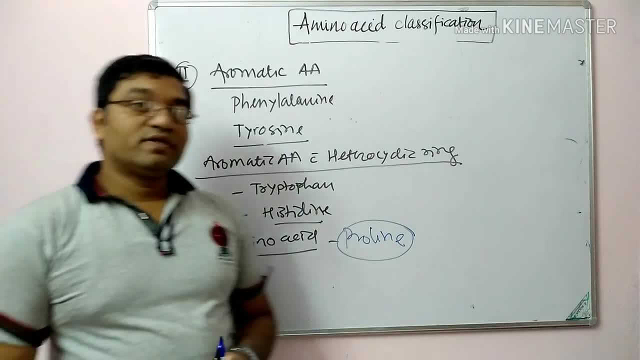 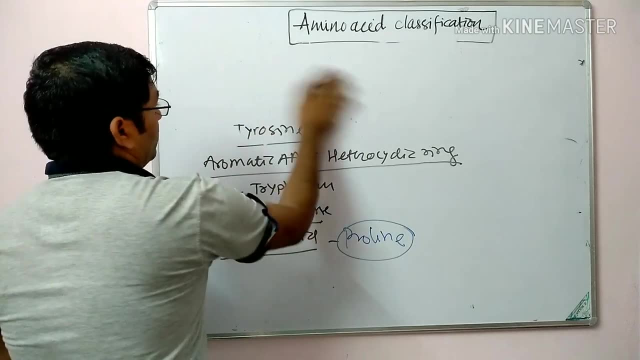 So this is the structural classification of amino acid: The first one with aliphatic side chain, the second, aromatic amino acids and third one is the immune acid. Now coming to the polarity, the classification based on the solubility or polarity. 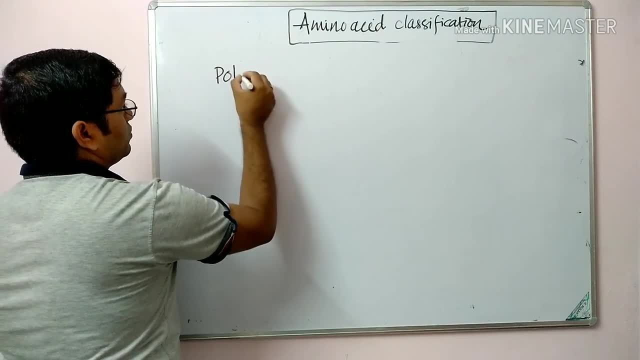 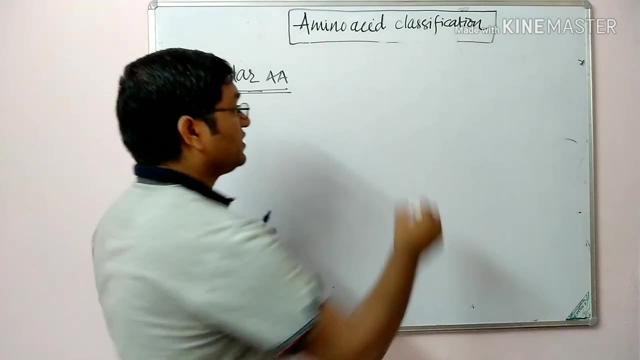 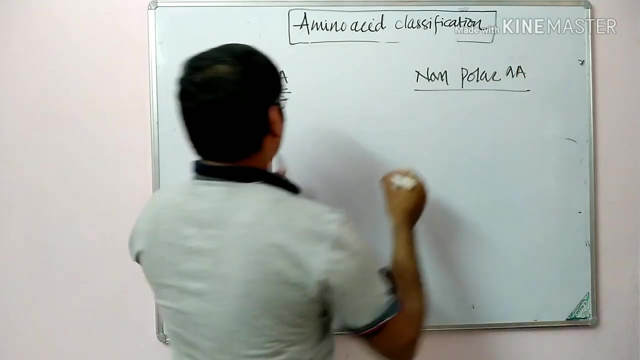 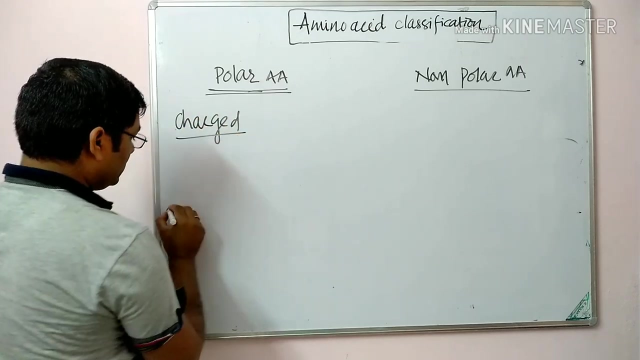 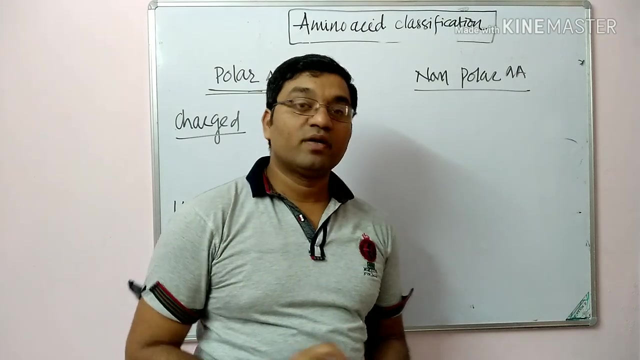 They are classified as polar Polar amino acids, Or you can say it as hydrophilic amino acids and non-polar amino acids. In these polar amino acids there are charged and uncharged. Of these, charged ones are very simple to remember. 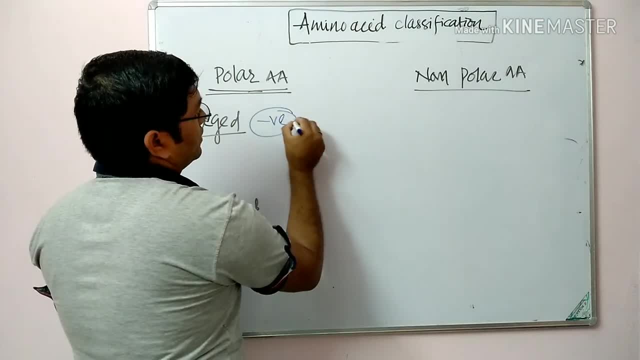 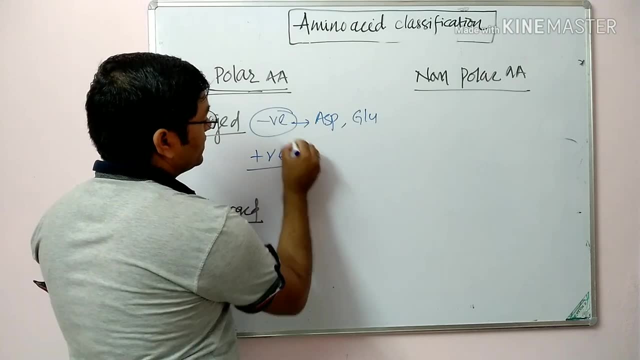 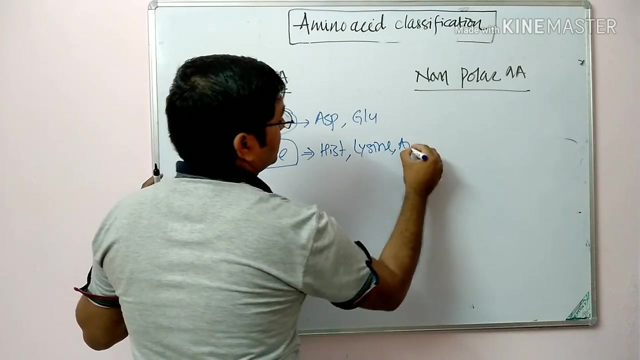 The charge includes the negatively charged, that is, aspartic acid and glutamic acid, And positively charged They are basic amino acids. That is, its basics are lye Means, histidine, lysine and arginine. So these are negatively charged acids. 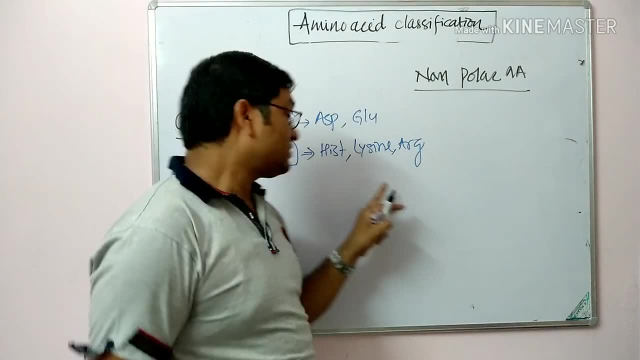 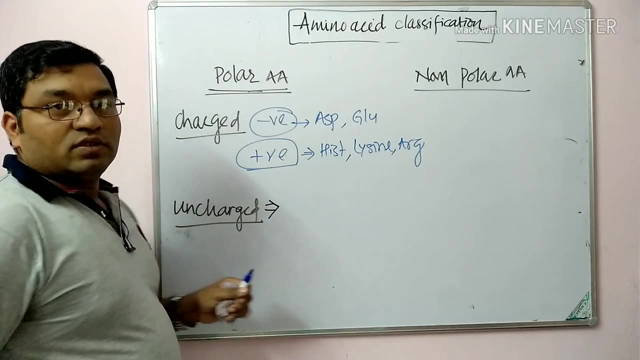 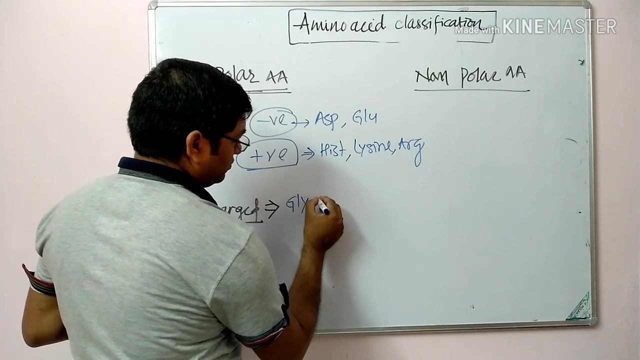 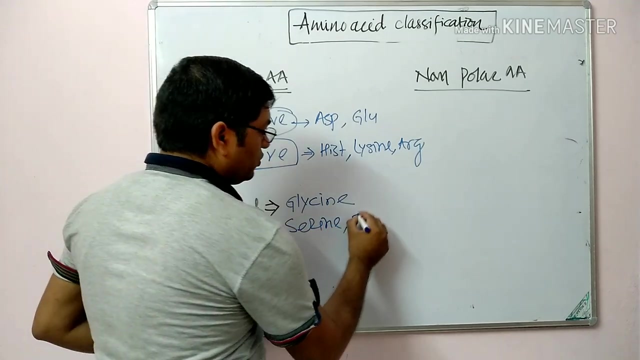 And positively charged basic amino acids, that is, histidine, lysine and arginine. Its basics are lye, Then in uncharged. In uncharged, it includes glycine, Glycine. Along with glycine, it includes serine, threonine, asparagine and glutamine. 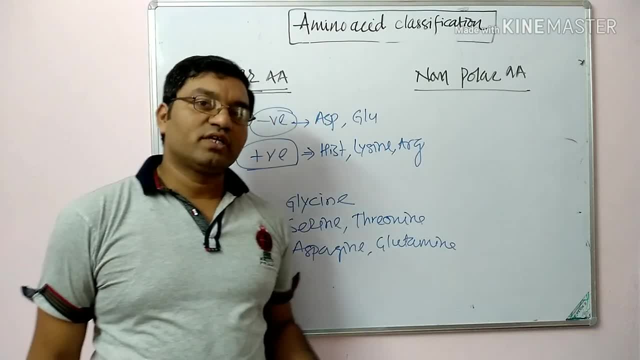 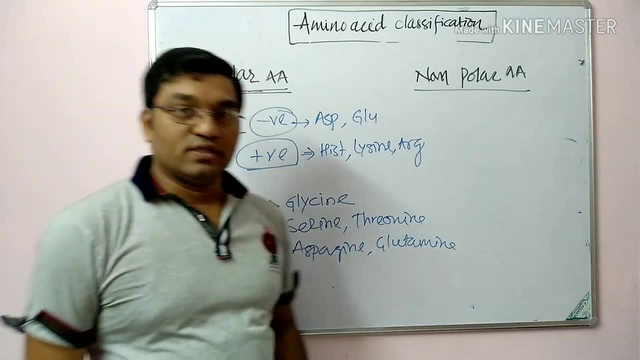 Remember two to three amino acids. if you want to write a short note in exam For entrance purpose, please remember all amino acids which belong to the uncharged polar amino acids. Okay, Coming to the non-polar amino acids, This especially includes the arginine. 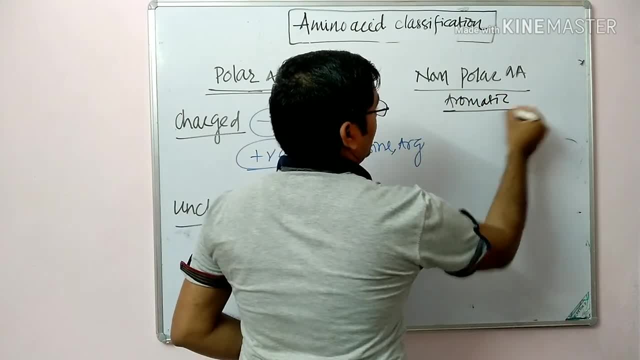 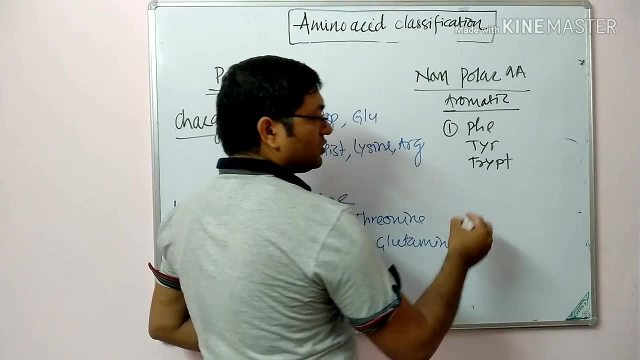 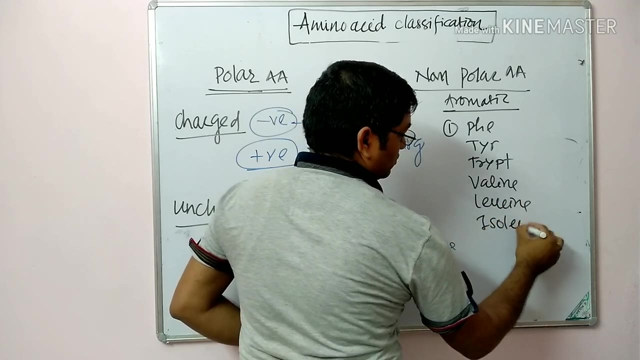 These are the aromatic amino acids. These aromatic includes phenylalanine, tyrosine, tryptophan. Then it includes branchin, that is, valine, leucine, isoleucine. It also includes methionine. 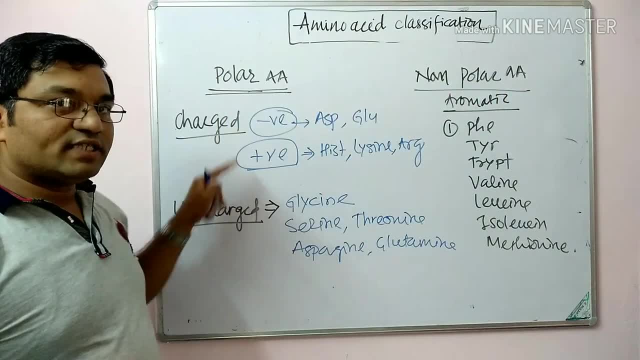 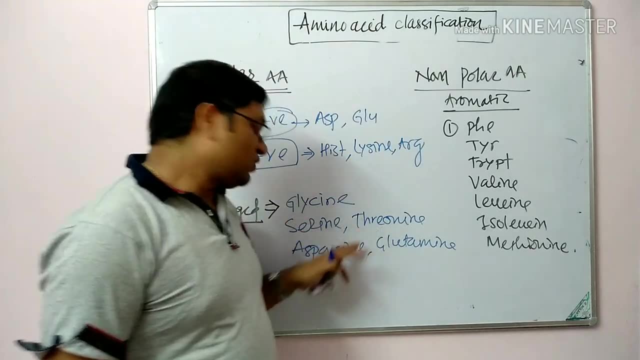 So these are the polar non-polar. Polar includes charged uncharged. In charged they are negatively charged. These are the acids Positively charged. they are basic amino acids. Then, uncharged, they include the glycine, serine, threonine and amino acid with amide group. 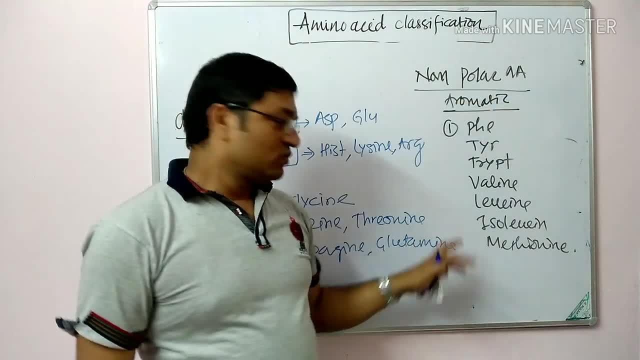 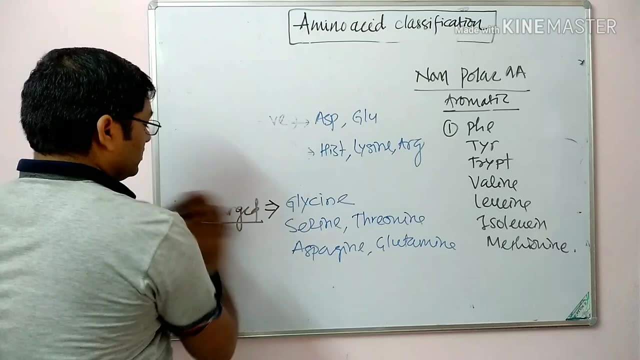 In non-polar amino acids. it especially includes aromatic and branchin amino acids, Along with methionine and alanine. So this is the classification based on the polarity. Now, coming to the nutritional classification Based on the nutritional requirement. they are essential and non-essential. 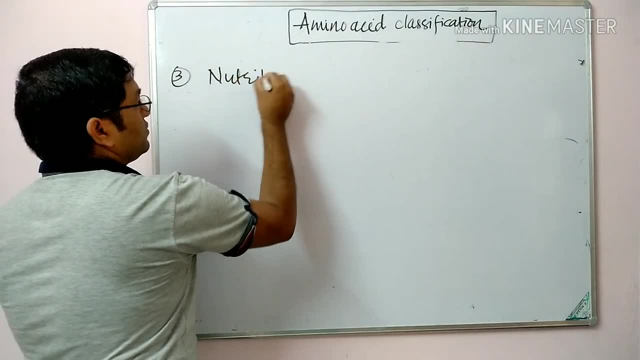 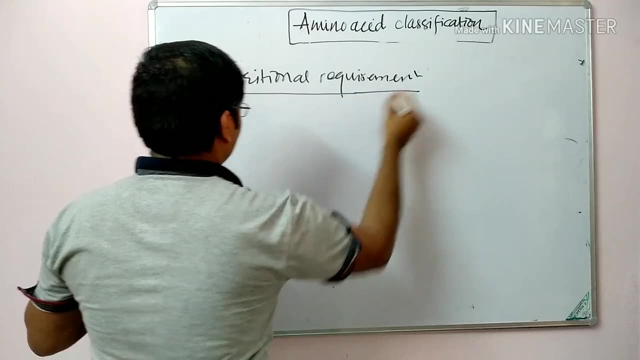 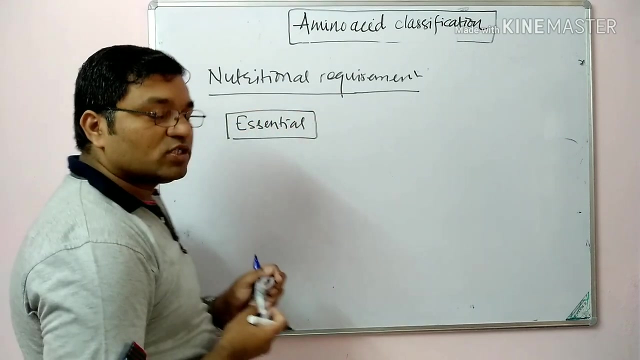 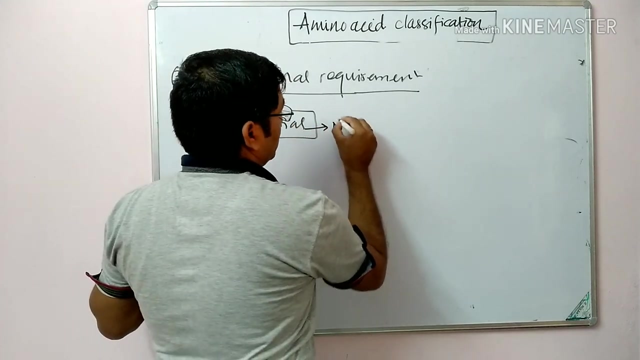 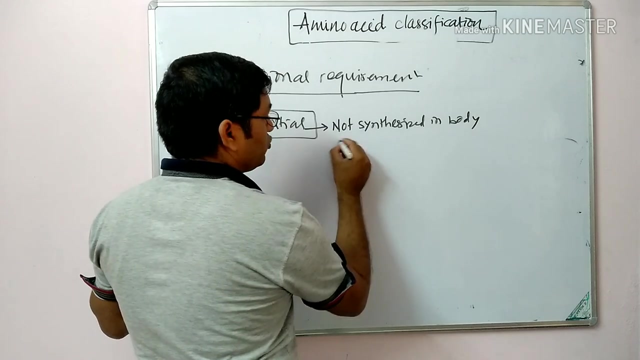 Third classification, based on the nutritional requirement. So again without quantification on the plausibility and the content, there are notwenty such reinforces of amino acids. It is that they are performed in acid, So this might be auto Em Yin In an inanimate form. they are intra-inanimate. 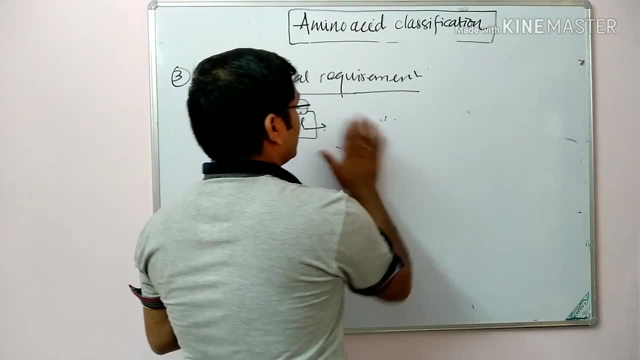 So they are classified as essential amino acids, Which means those amino acids which need to be supplied in the diet. they are not synthesized by the body. They are known as essential means: not synthesized in body has to be supplied in the diet as essential amino acids and other ones. they are known as non-essential amino acids. So they are very simple to remember. There are two types: essential and non-essential. in between, There is semi-essential. also, There is mnemonic for essential amino acid that is mat will fly. This is very famous mnemonic, that is mat will fly. There are 10. 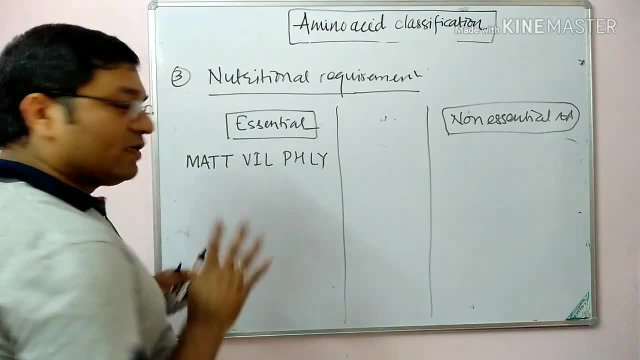 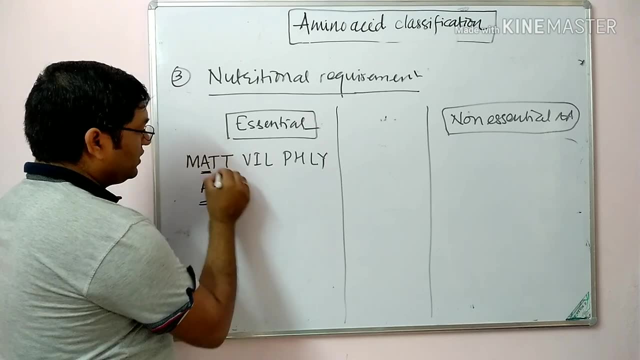 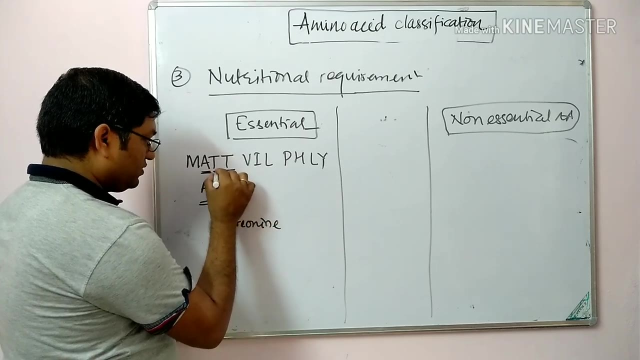 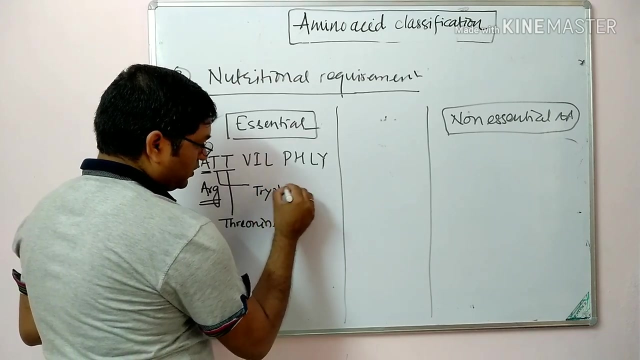 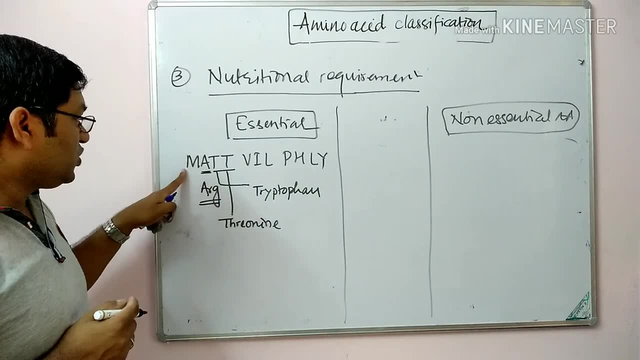 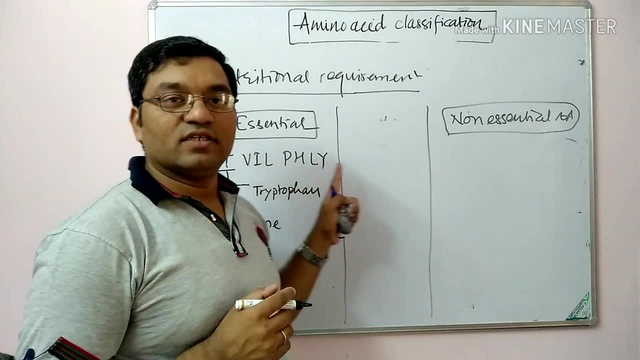 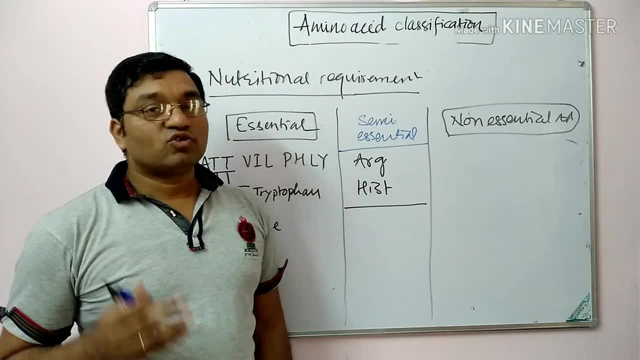 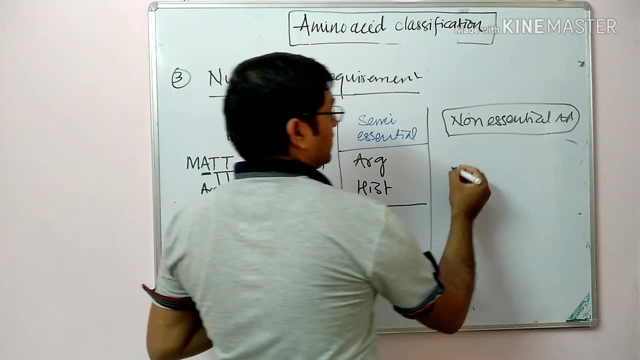 demand increases, for example, in pregnancy and growing children. there it has to be supplied in the diet. that's why they are known as semi-essential amino acids and remaining all amino acids, remaining all amino acids. they belong to the non-essential amino acid, so this is based. 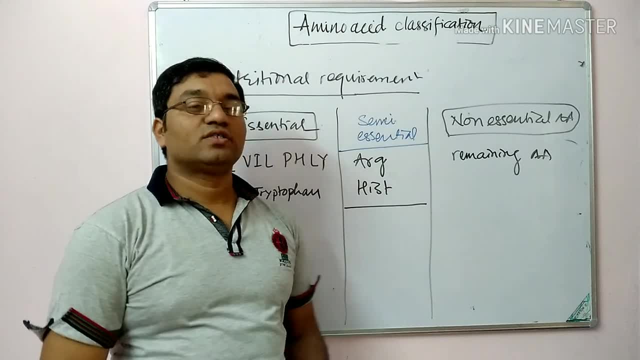 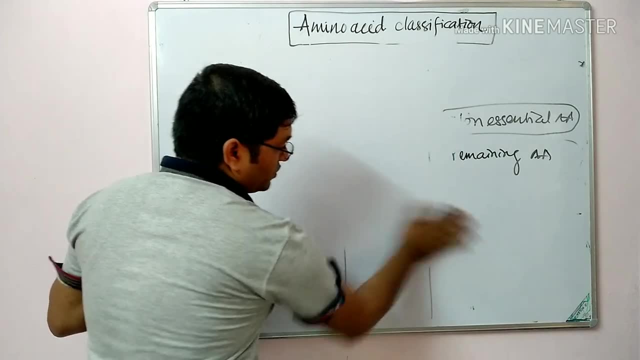 on the essentiality. they are classified as essential, semi-essential and non-essential amino acids. coming to the fourth classification, that is, metabolic fate. it is very easy to remember: the amino acid which gives glucose- they are known as glucogenic. the amino acid which gives ketone or fat, they are known as chlotogenic amino acids- and which gives both: they are known.